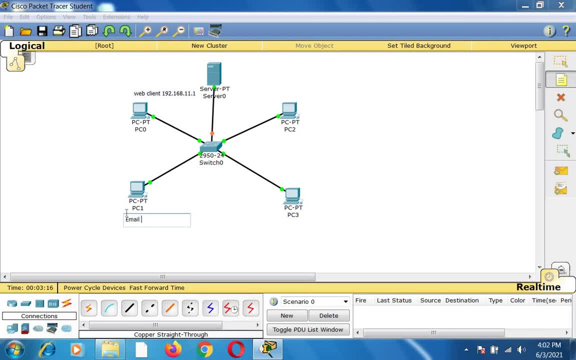 For PC1, I am naming it as email client 192.168.11.2.. So for the PC2, I am naming it as DNS client 192.168.11.3.. And for PC3, I am naming it as FTP client 192.168.11.4.. 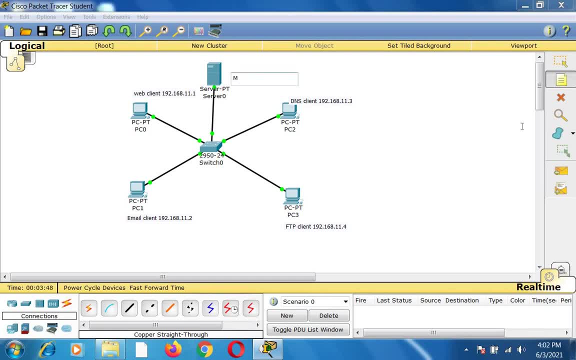 And for the server, I am naming it as multi server And the IP address is 192.168.11.4.. And the IP address is 192.168.11.3.. And the IP address is 192.168.11.4.. 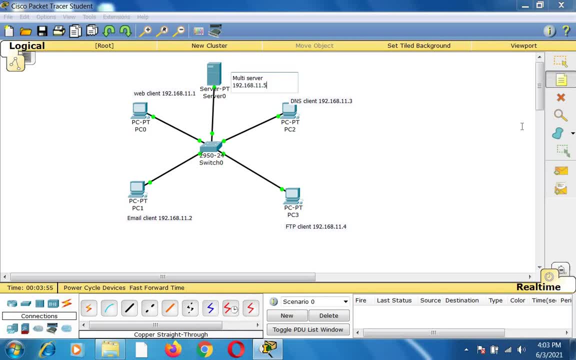 And the IP address is 192.168.11.4.. con for the depth. So I have typed: ok, 192.168.11.5. okay, so what i have done is i have created, i have given the names for all the nodes. 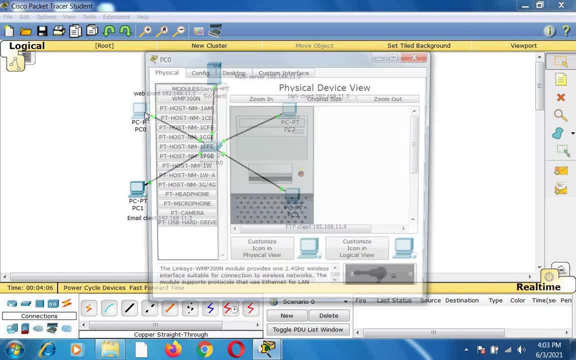 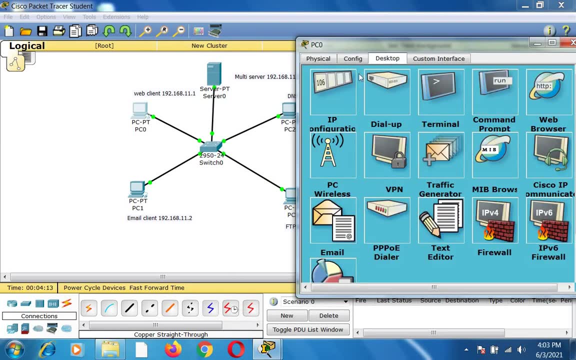 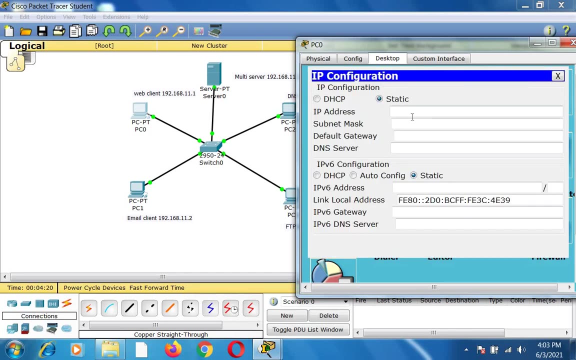 now i will click these into these nodes and i will configure the ip address. so when i click this pc01, i'll get this dialog box. under this, i'll click this desktop option. under desktop option, you have several options are there. i am going to click this ip configuration and then i am going to configure. the ip address of pc0. so pc0 ip address is 192.168.11.1 and i am also configuring the dns server. the server address is 192.168.11.5, so we have given the ip address for the server to be 192.168.11.5. 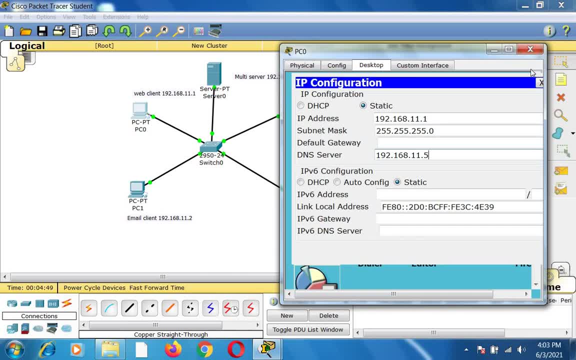 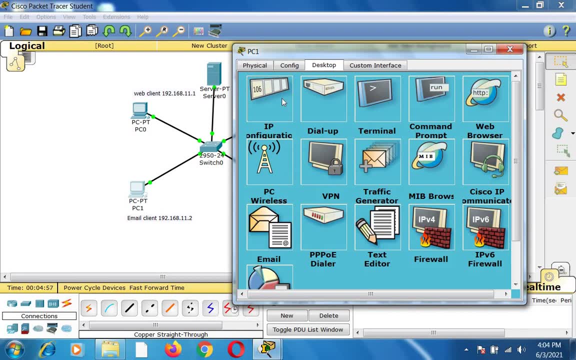 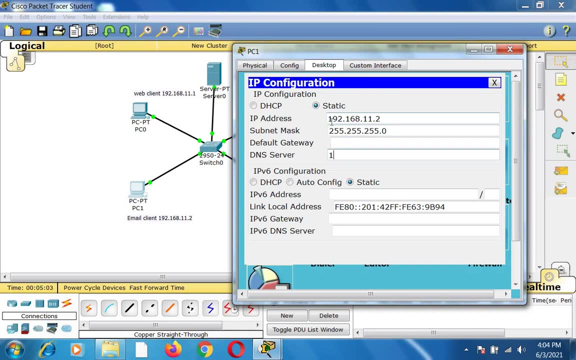 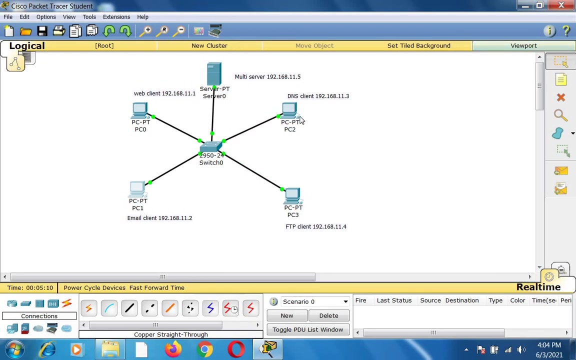 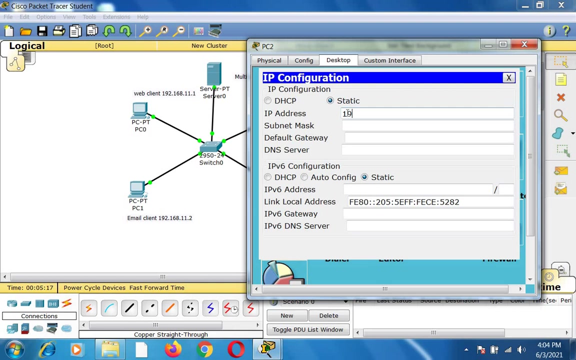 that i am configuring to the pc0. likewise i am creating, i am configuring, configuring other nodes also. so pc1 ip address 192.168.11.2 and server address is 192.168.11.5. pc2 desktop ip configuration. ip address is 192.168.11.3. dns server is 192.168.11.5. 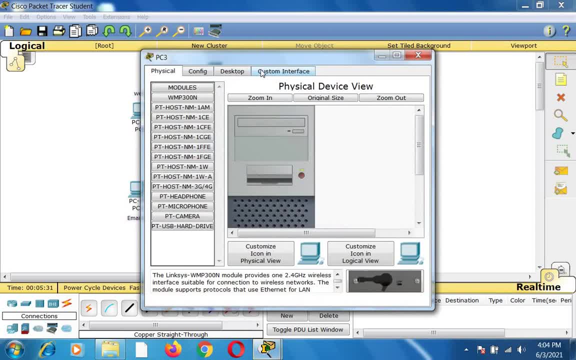 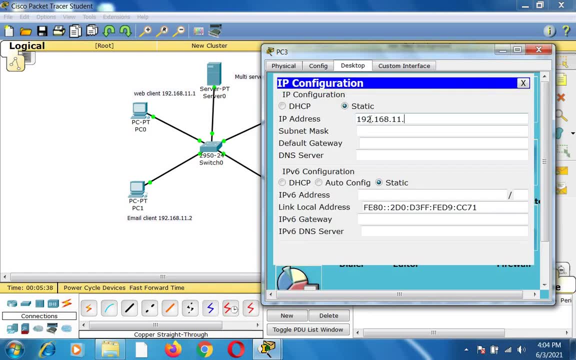 pc3 address. one ip configuration: 192.168.11.4- 192.168.11.5. last i am going to configure the ip address for the pc0 ip address: 192.168.11.3. dns server is 192.168.11.5. 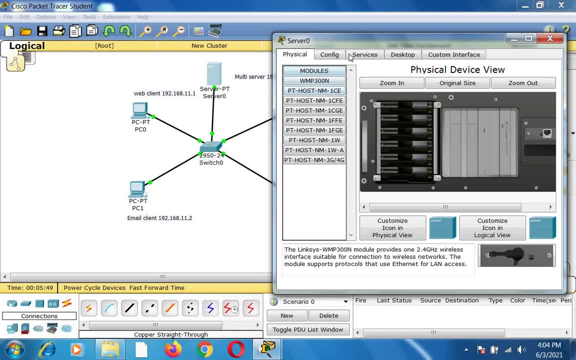 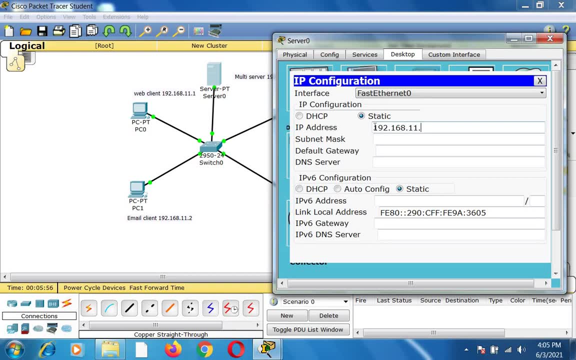 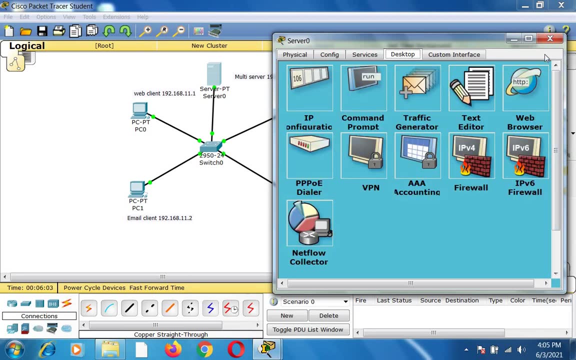 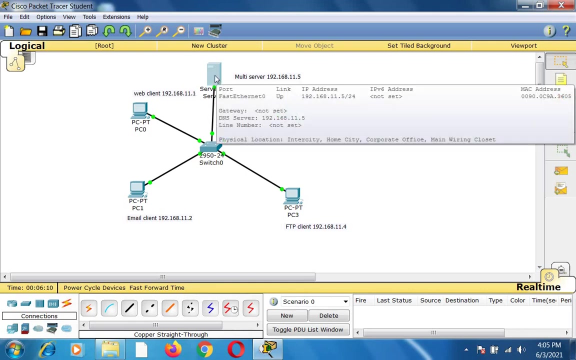 i am configuring the server address. server address to be go to desktop ip configuration. ip address: 192.168.11.5- 192.168.11.5. okay, so i have configured the ip address and also server address for all the clients in server nodes. so now. now what i will do is i'll go to the server. 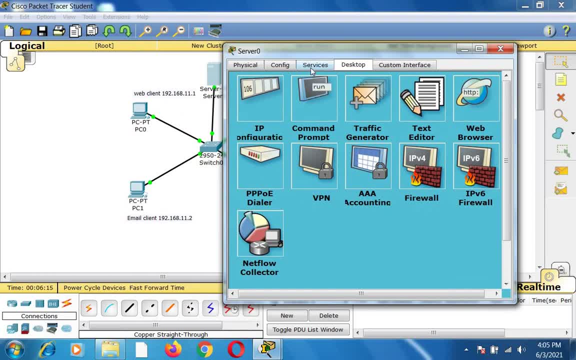 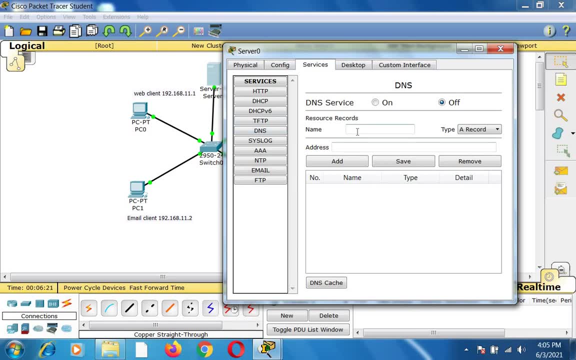 multi server and under this i'm, i'll go to the server and i'll go to the server and i'll go to the services option. in the services option, i'll go to this dns domain name system and i'll create a new recorder. so for this, i am going to give the record to be googlecom and the address for this. 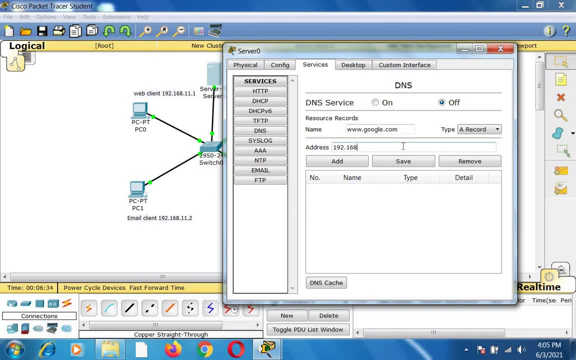 googlecom is 192.168.11.5. okay, i am adding this record into this domain name system. i am switching on this domain name service. okay, domain name service and i'm adding this record. googlecom address is 192.168.11.5. okay, add this record now. so this record is added. then go to. 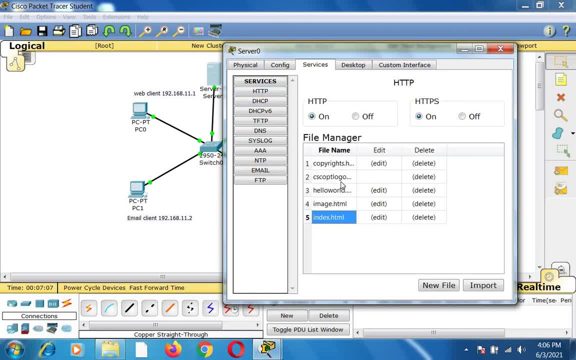 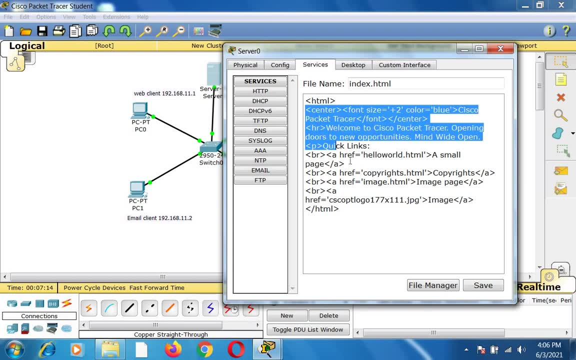 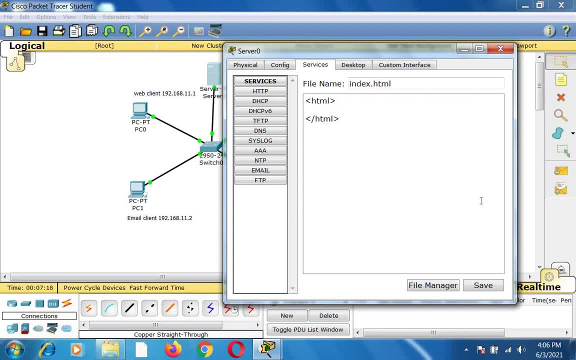 content is there. you delete the content of this html body, of this html. now you can give your own content. i am going to give it as welcome to my page. save this file. it will ask whether you want to overwrite. ok, give as yes. so now what i have done in the server. go to server. i have gone to. 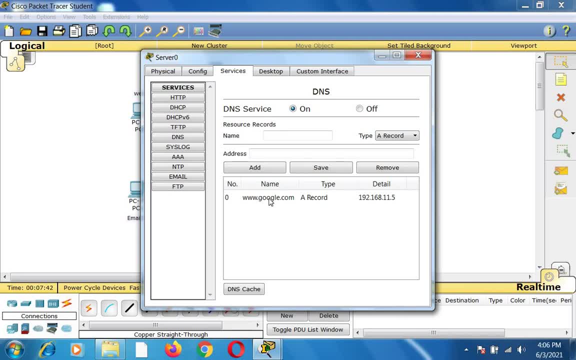 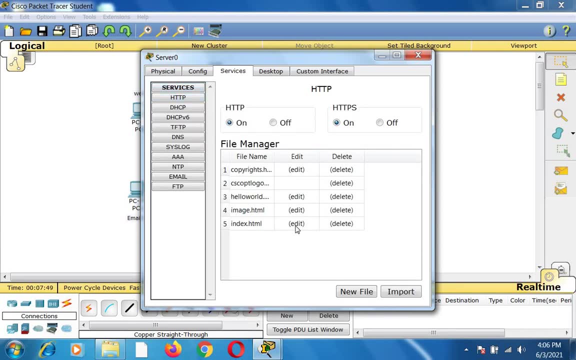 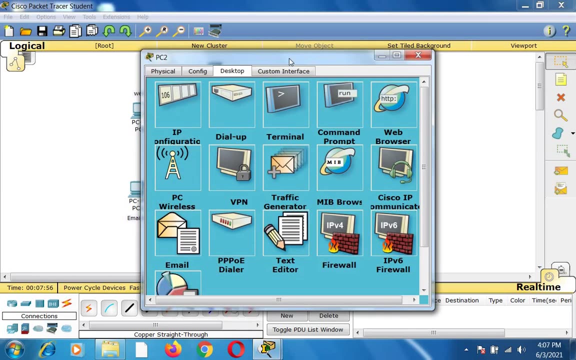 dns and i have added a new record. i have given the the googlecom rdp address and then i went to http. i went to http and i have changed the index page. ok, so now i will go for this domain name service client. click on this domain name service client. go to command prompt under this. 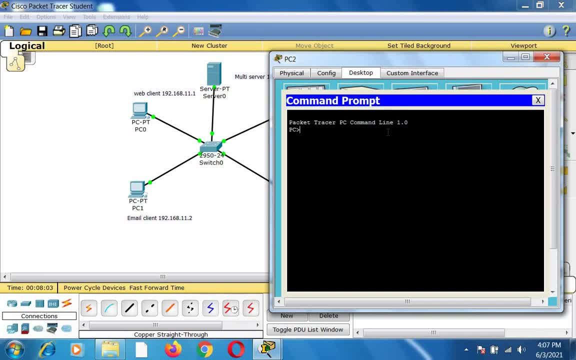 desktop. you have a command prompter in the command prompt. when you click this command prompt you will get a command prompt. so in this you type ns, lookup, lookup, googlecom. so this command will tell you whether you can able to connect with the server or not. so 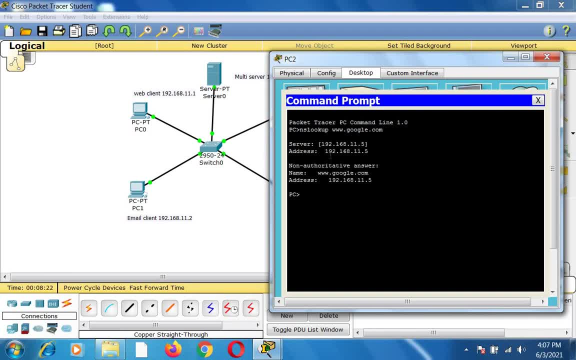 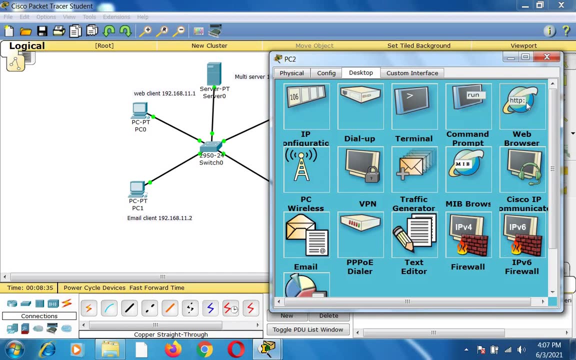 when you click this, when you type this command, it says that the ip address of this googlecom is 192.160.11.5. this command says that the client- dns client- can able to connect with the server and can able to resolve the ip address. ok, now this is working. now again you can go for web browser. 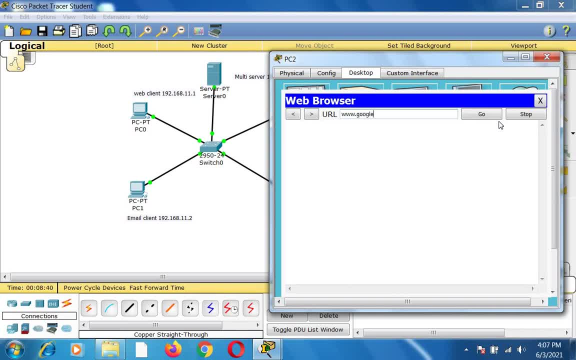 and in the url you can go for the web browser and in the url you can go for the web browser and, additionally, you can give the google address. so when you give this google address, you should able to get the page, what you have typed at, so i should able to get the welcome. 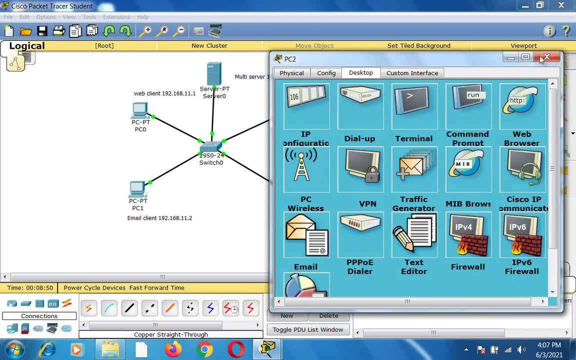 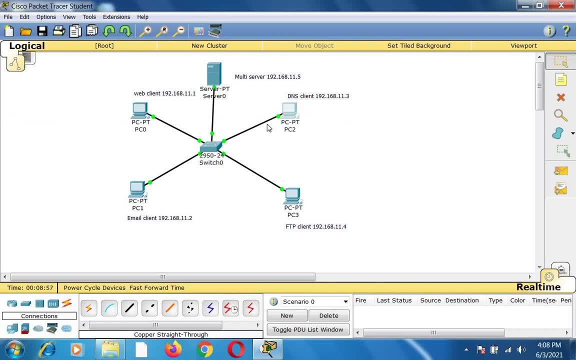 to my page. yes, it is also working. so we have worked this domain name client. so what we are doing in this video is i'm going to tell you how all these clients can be connected with the server and how tcp adp performance can be measure. that is what i am going. 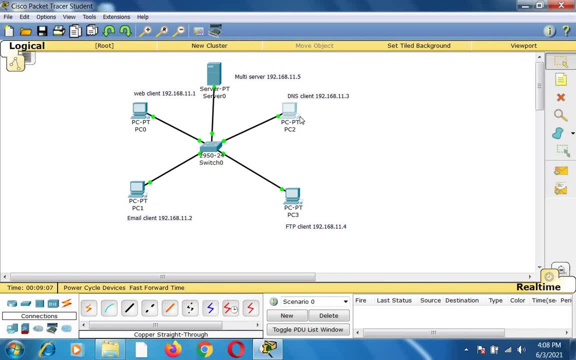 to explain to you. so i have explained to you about domain name client, domain name systems where i have highlighted or written this information. ok, you can first go back to the desktop spoofing name system. so where i have set the configuration in the server and, using this client, i can able. 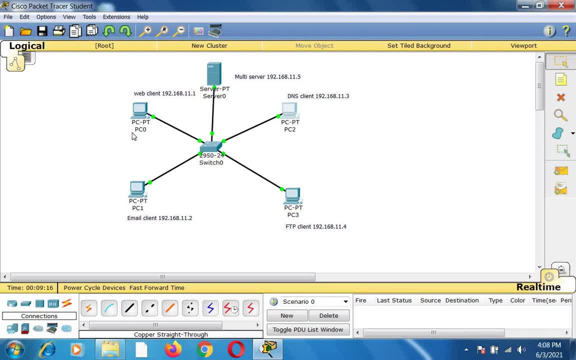 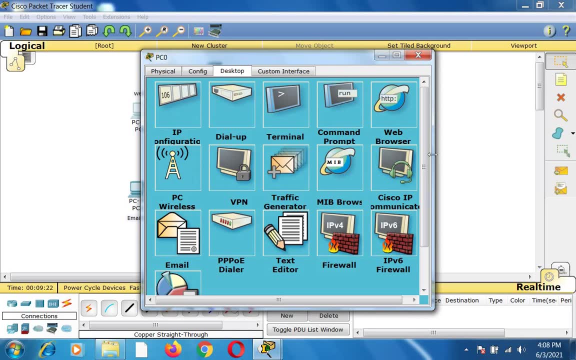 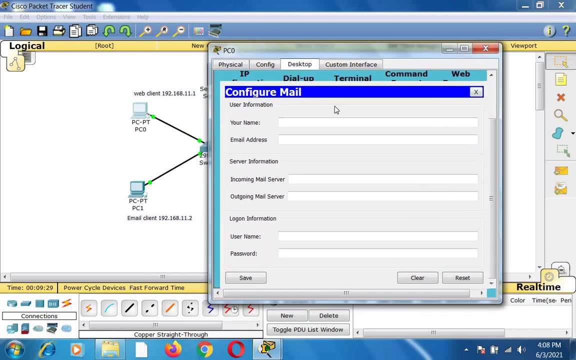 to resolve the domain name. next we move on to the web client and email client. okay, so for the web client, go to this web client and you have several option in this desktop. under this you have an option called email. so click this email, okay, and in when you click this email, you will get this. 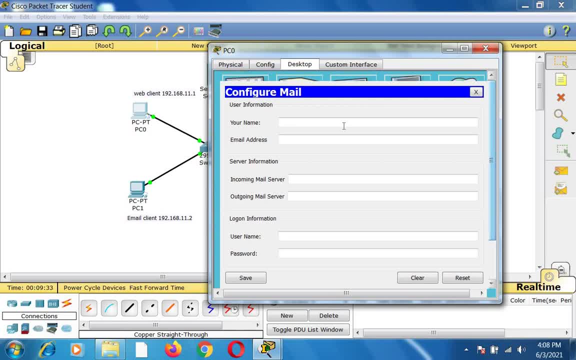 dialog box: configure mail. so configure mail you can. it is asking your name, so i am giving my name, my. i am giving my name, the email address priti at gmailcom incoming mail server. i am giving this the server ip address: 192.168.11.5. outgoing mail server address is also the same ip address of the. 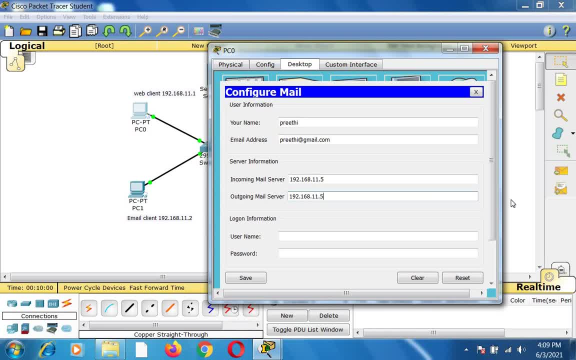 server: 192.168.11.5, 192.168.11.5, 192.168.11.5, and it is asking the login information username. i am giving my name. password is cisco. okay, so something. i have given the password, so i am going to save this option. so you are giving the. 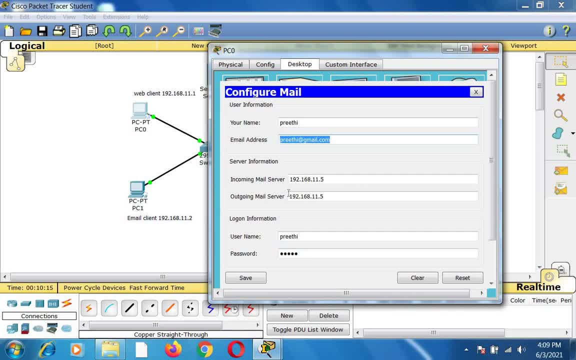 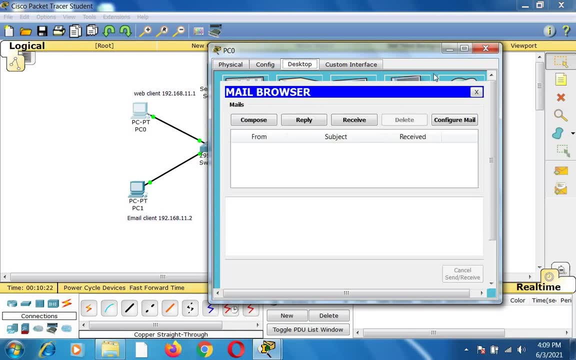 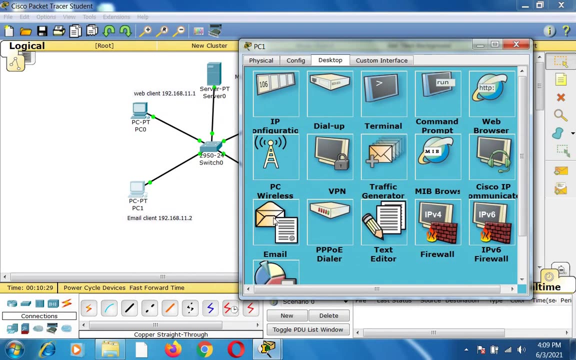 configuring your mail. you are setting this email address and it is asking for the incoming mail server and outgoing mail server. it is asking the username and password. okay, save this option. that is what you have to do. it in web client, then go to the email client, also in the email client, similarly. 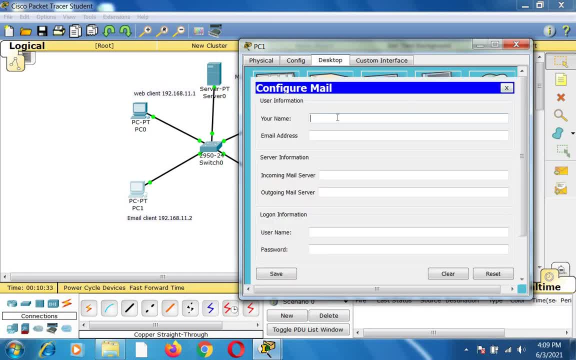 you go to email option. under this email you create some other mail address. so i am creating the another mail address. okay, venkatesh. venkatesh at gmailcom incoming mail server. i am giving 192.168.11.5 and 192.168.11.5, okay. username password is cisco, okay, so i have created two mail address, one in the. 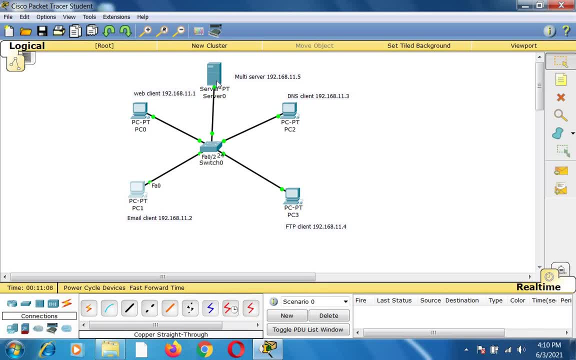 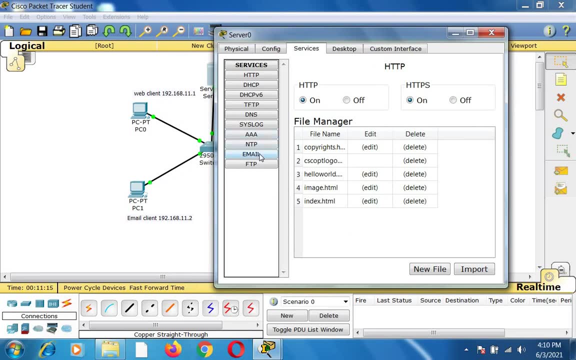 web client, another one in the email client. now again, i'll go to the multi server. in the multi server i'll go for the services in the services. i'll have email services. click on this email services, switch on this smtp servers and pop 3 servers and i'll go to the multi server and i'll. 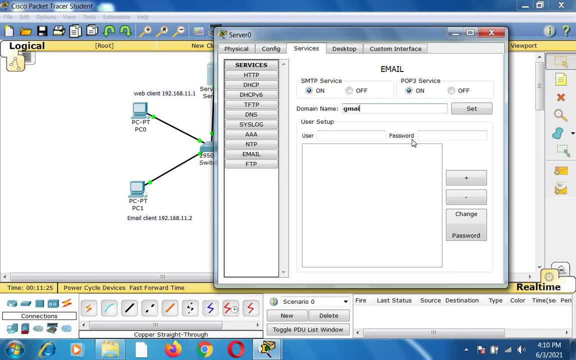 create the domain name. under this domain name, i'll create this as gmailcom. okay, give this set option and you give the username and password. so we have created the email address for priti and the password is cisco. likewise one more user. i have created venkatesh. password is cisco, okay. 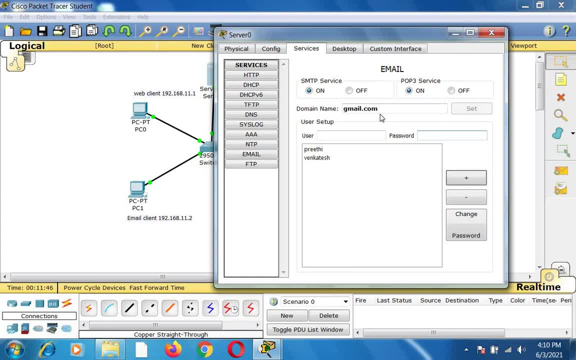 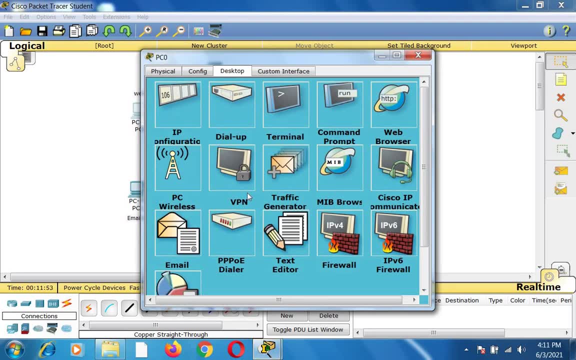 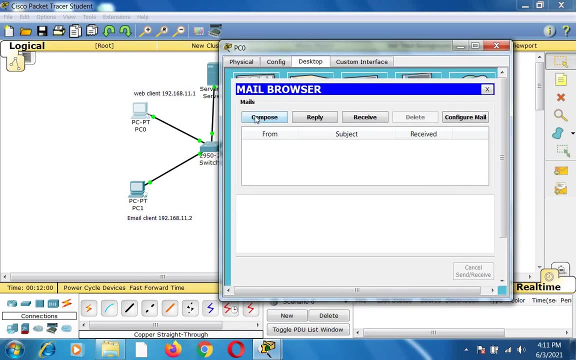 so i have created two email address under the domain name gmailcom. okay, so now what we'll do is that's all you have to do it in multi server. go to web client. now go to again email. try to send email from pc0 to pc1. okay, that is what we are going to do it. so i'm clicking this pc0, then mail. that is like email compose. go to compose mail. give the email address venkatesh at gmailcom. subject: i'm giving hi. in the body of the message i'm giving hello. okay, give send option. 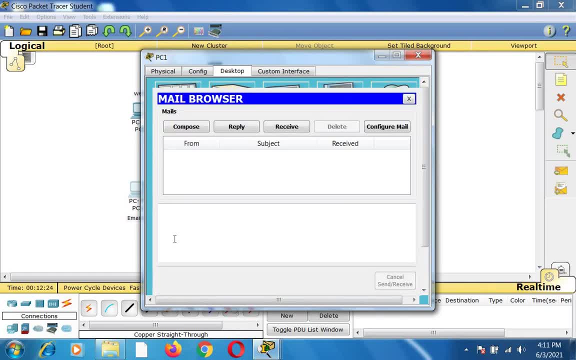 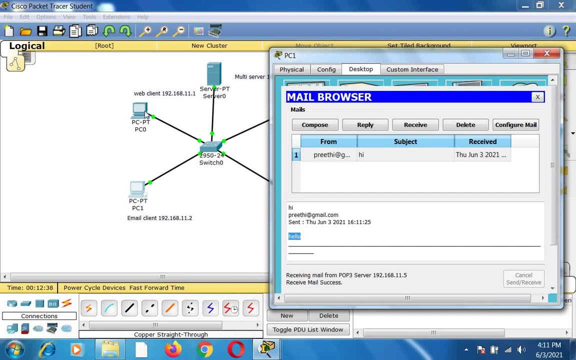 now i'll go to pc1, go to this email. you give it as received. so once if you give receive, you can able to get it in the inbox. when you click this inbox you can see the message hello message in this. so what happened over here is i can able to send the mail from pc0 to pc1. okay, so i can also send. i can also check whether i can able to send a message from pc1 to pc0. so what i'll do is i'll give compose again. so i'm trying to check whether i can able to send a message from pc1 to pc0. so what i'll do is i'll give compose again. so i'm trying to check whether i can able to send a message from pc1 to pc0. so what i'll do is i'll give compose again. so i'm trying to check whether i can able to send a message from pc1 to pc0. so what i'll do is i'll give compose again. so i'm trying to check whether i can able to send a message from pc1 to pc0. so what i'll do is i'll give. 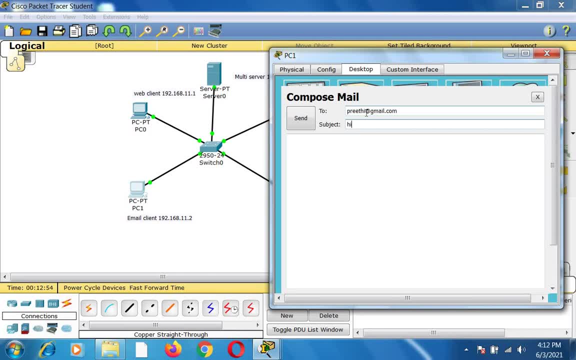 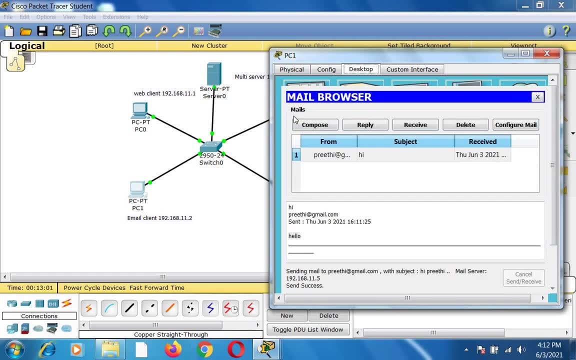 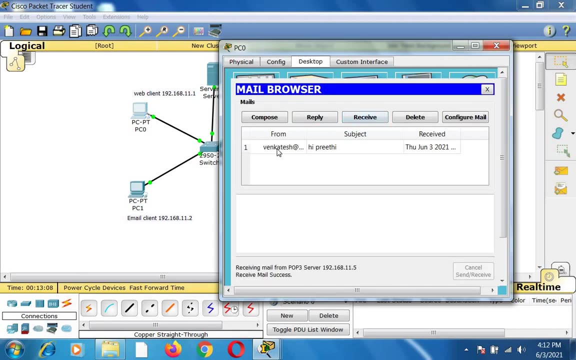 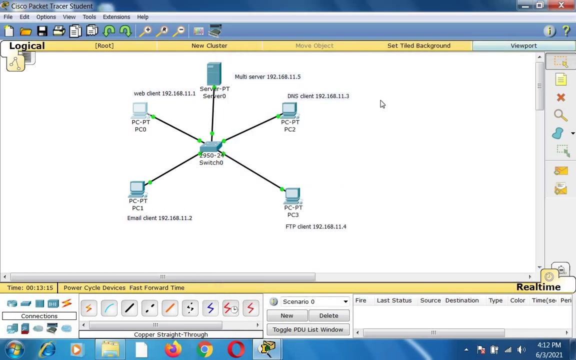 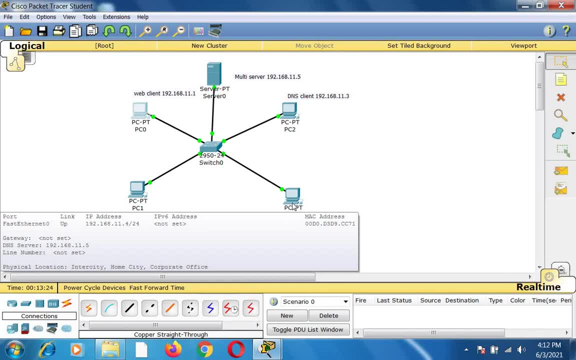 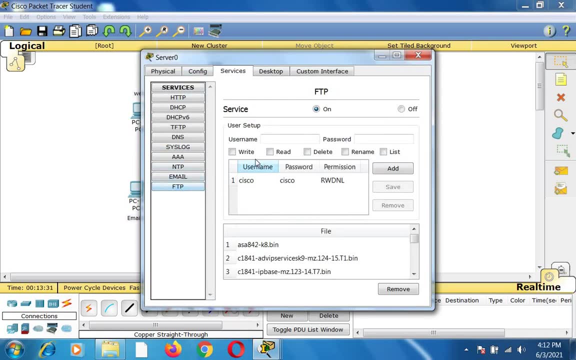 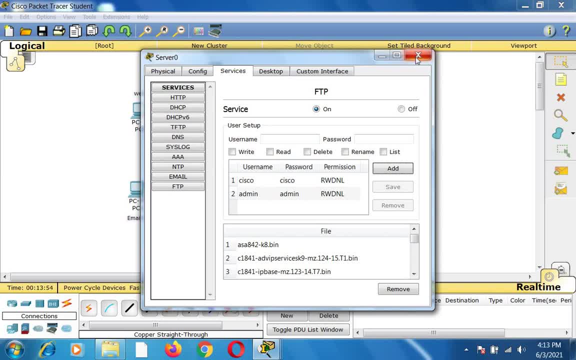 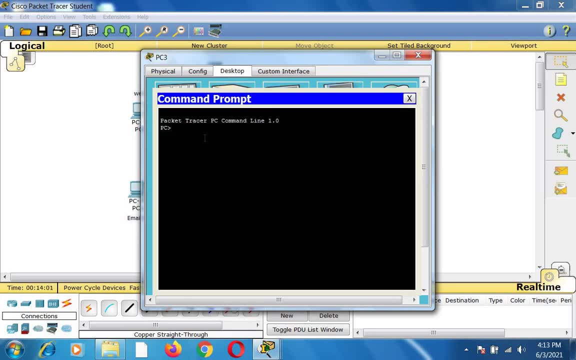 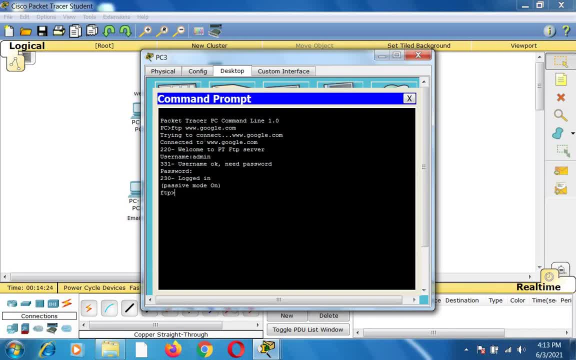 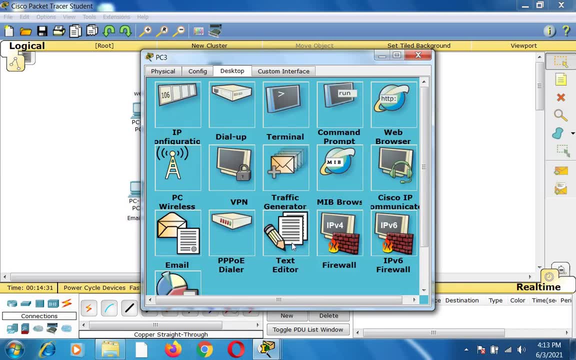 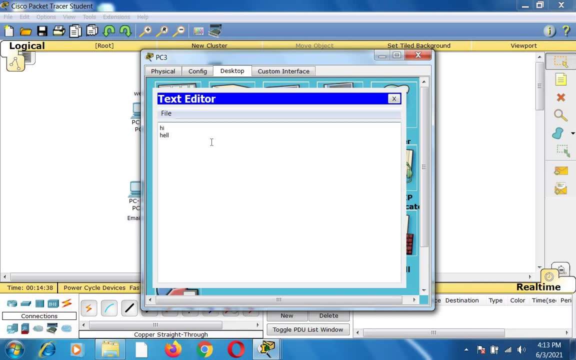 so when you type this ftp command prompt, you will get the ftp command prompt. so what you can do is: i am, i have, i have opened in this pc3, right, so i can go to a text editor. you have one more option called text editor, so text editor. you can type something. hi, hello, how are you okay? so try to. 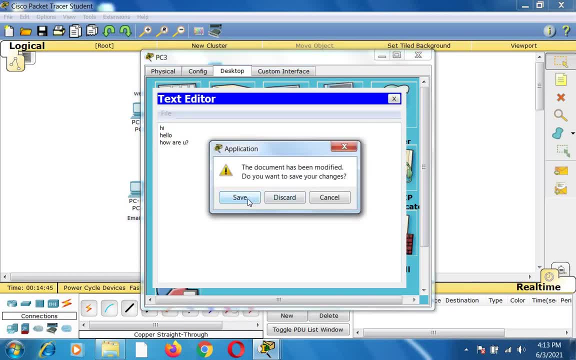 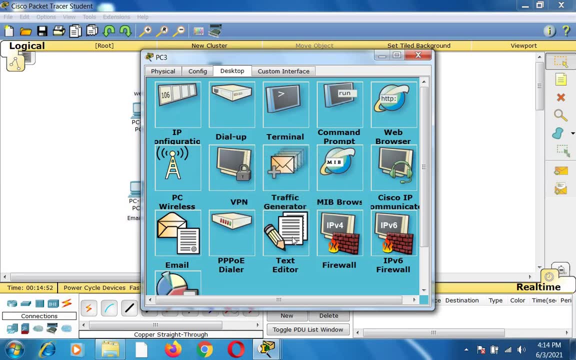 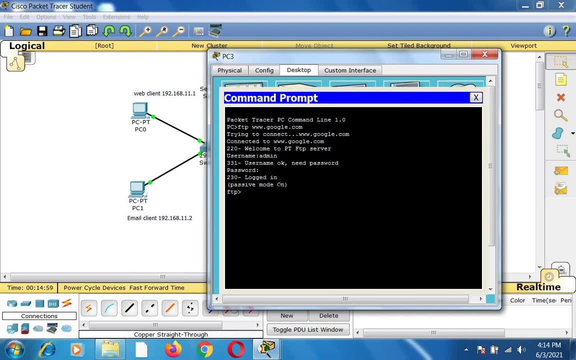 save. when you close this file it will ask for save option. do you want to save? save this file under the name text test. okay, give this as okay command. so i have created one file in pc3. okay, go to this command prompt again. now i want to put this. i want to send this file to the server. 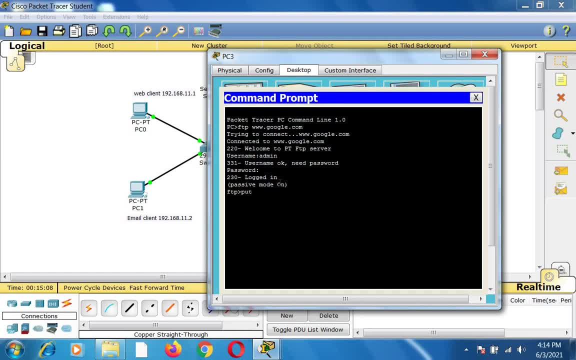 so for this i can use a command called put, put test dot txt. okay, this is a command for transferring the file from the current node to the server node. so when you give this, okay, so i have created one file in pc3. okay, go to this command prompt again. now i want to 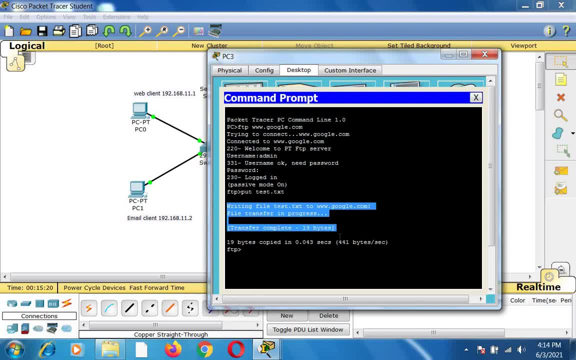 option. it is saying that writing the file to the googlecom. so it has returned this particular file. it has transferred the file to the server. so you can use directory option to see whether it is whether your file is there or not. so you can see this. when you give this directory, you can see the 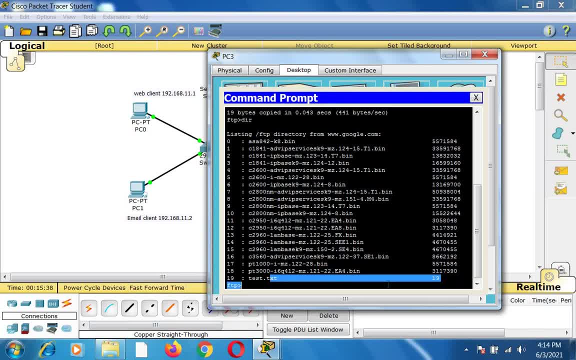 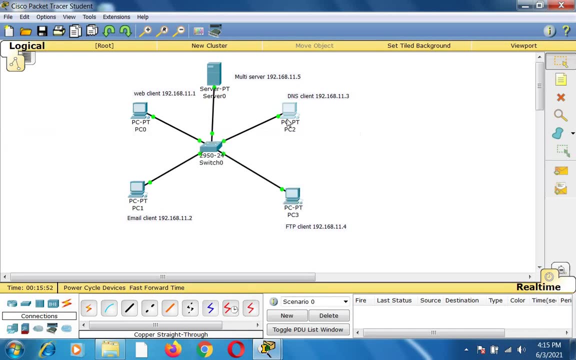 file test dot txt. in the 19th file it is listed. your file has been listed, okay, so this is what we have. this is called uploading the file. you are uploading your file into the server. so now what we will do is: we will try to this. we have done in ftp client, so we open in dns client. 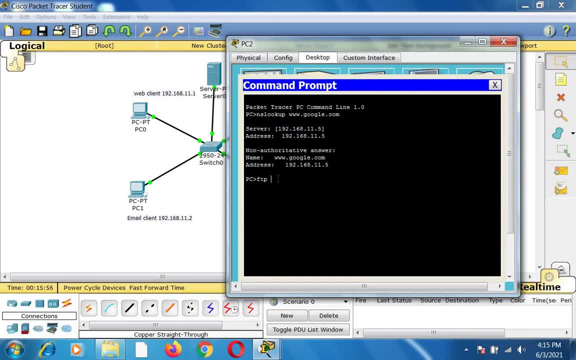 in the command prompt. go to this ftp- ftp- googlecom. you try to connect with the server address, give the admin and password. okay, now you will get your ftp command prompt. so now we have. we try to download the file. so for downloading the file you can, you can use an option called. 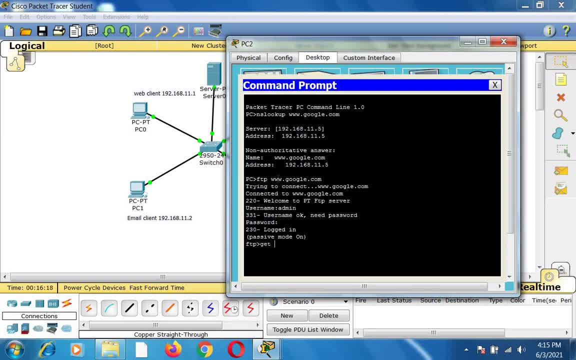 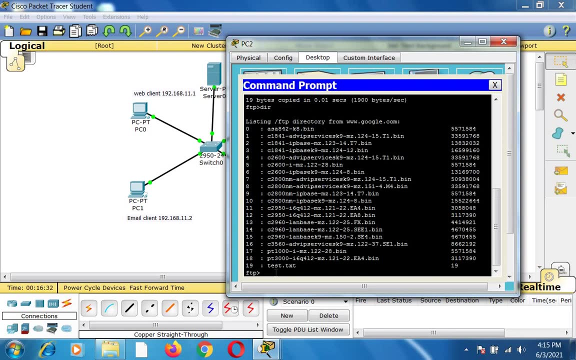 get, get test dot txt. okay. so when you give this text dot txt, it is reading the file from the googlecom, it is transferred. that file has been transferred to this, to this particular client. so when you give directory option, this directory, this current node, will also it will get the file. this is how you can. 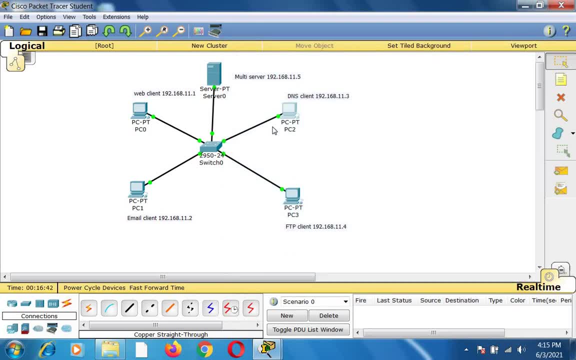 able to transfer the file from one client node to the another client node. so that's all. so now we have configured all the nodes. I hope that you have seen this video. I hope you have learned how to do this web client and email, how to send mails between the client nodes. we know how to solve the domain name system and we know how to get and also put this, transfer the files, upload and download the files using file transfer protocol. now you click this option. 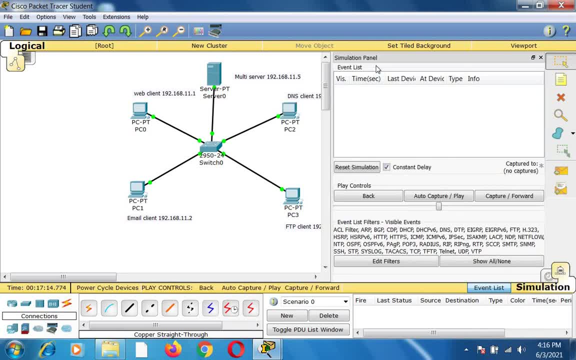 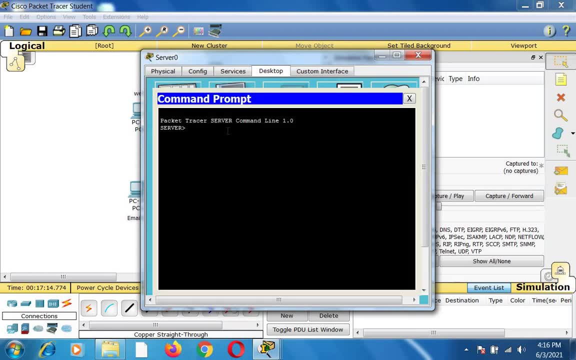 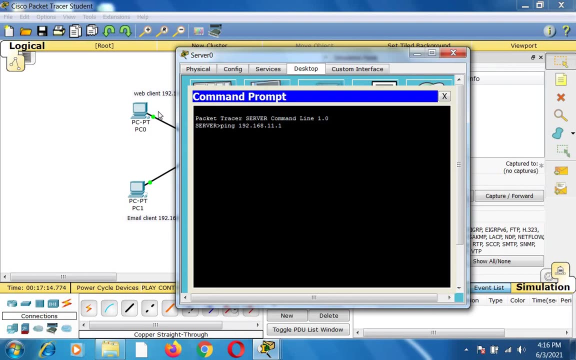 called simulation mode. when you mode, you will get this simulation panel. so what I will do is I'll click the server, go to desktop and I'll click this command prompt. I'll type: ping 192, dot, 168, dot, 11.1. I am trying to connect with the 11.1. okay, click so many. click this. 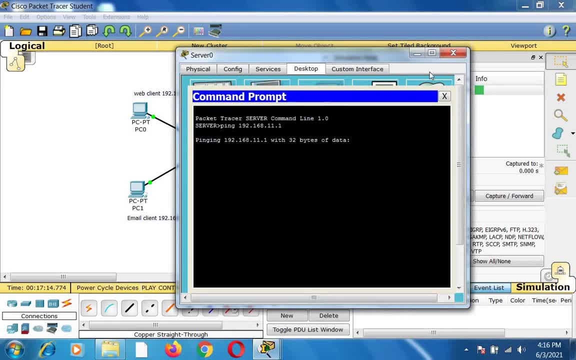 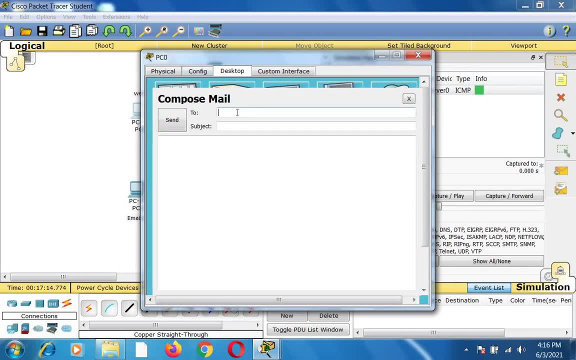 I'll get one packet over here, okay. next I'll go to this and click this email. I will click this compose. I'll type Venkatesh at gmailcom. subject: hi hi sender. okay, so you can see this to TCP packet. packets have been the have been.